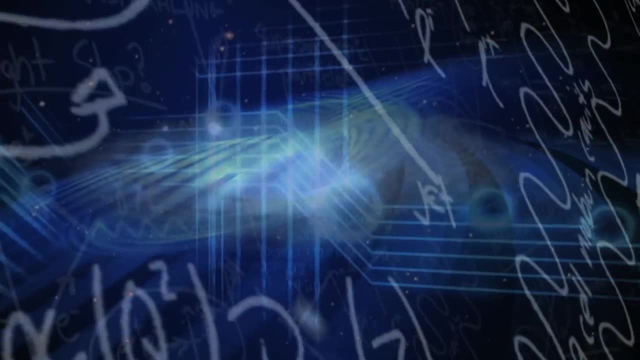 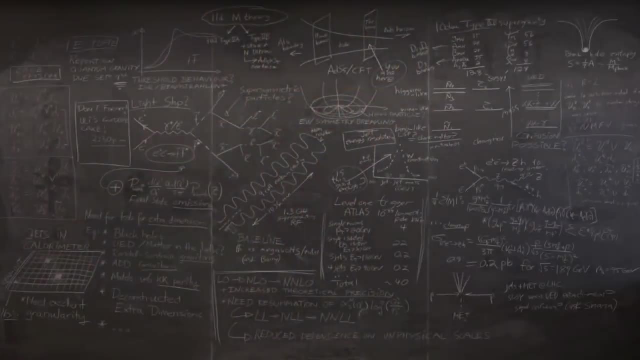 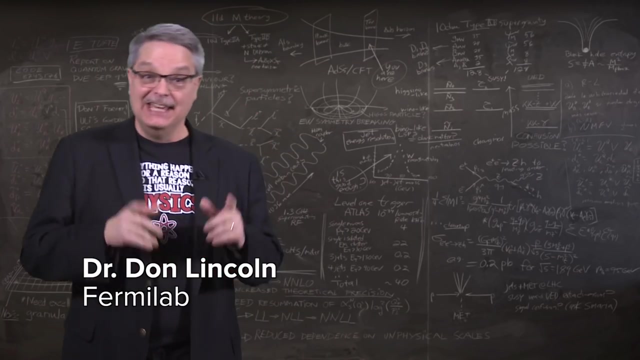 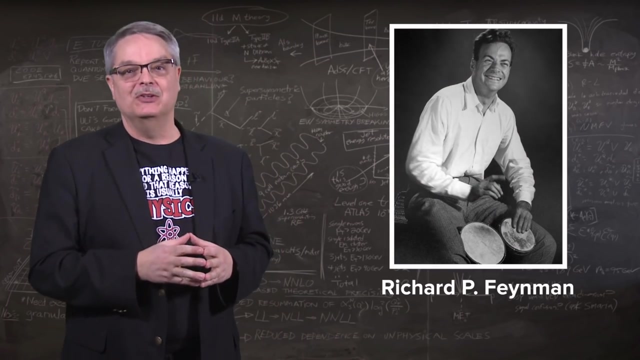 Every so often, a scientist is born who is so brilliant and so charming that they become a cultural icon. Now, I know that you thought I was talking about myself- well, because I get that a lot, but actually I was talking about Richard P Feynman, who is definitely 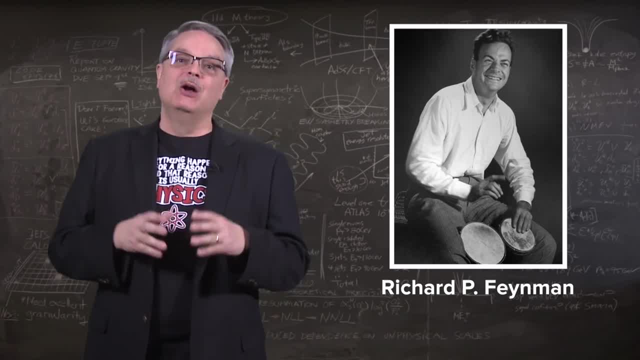 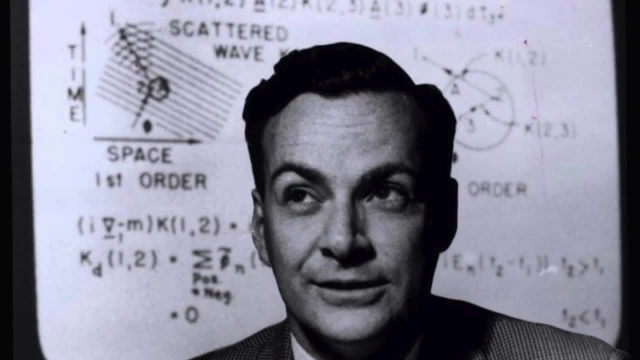 one of the coolest scientists of the 20th century. While stories abound of his interest in picking locks and his fondness for having a good time, it is in the realm of understanding the quantum nature of matter and energy that he made his real impact. 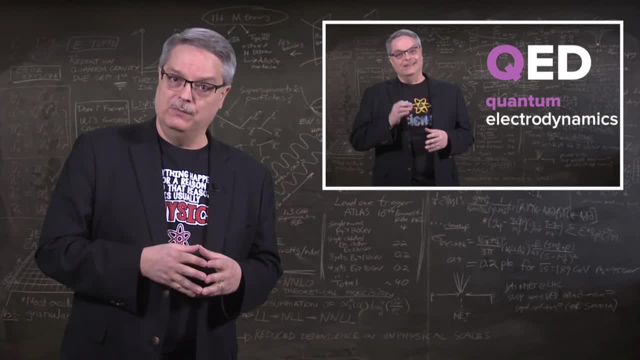 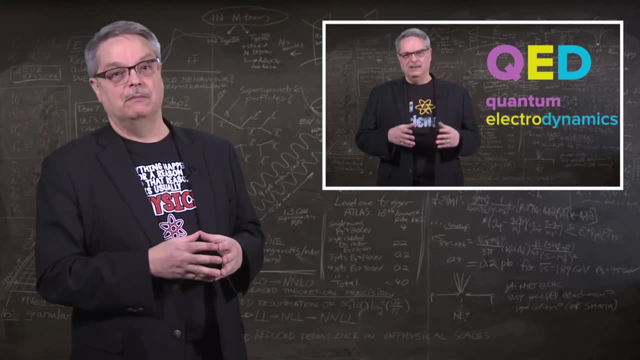 I tell the story of quantum electrodynamics in another video. In this video I want to talk specifically about his contribution to how modern physicists calculate how particles scatter. Now Feynman can't take all the credit. He shared his Nobel Prize with Julian Schwinger. 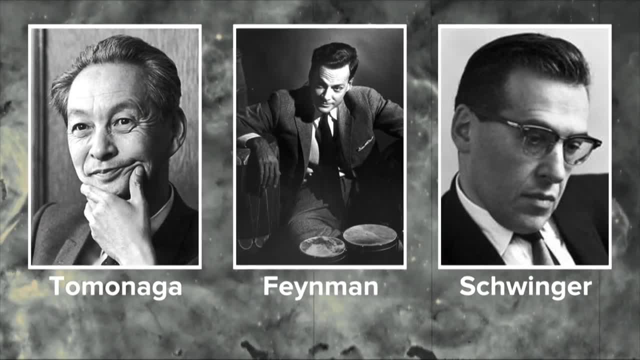 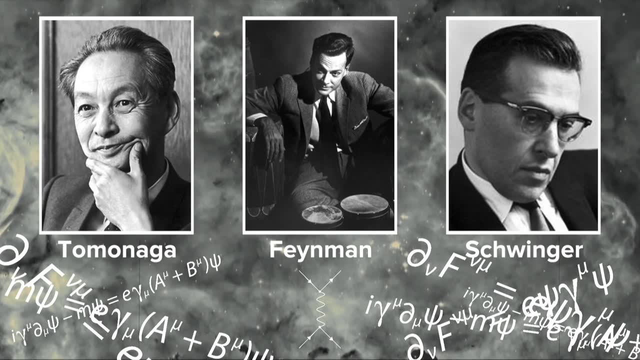 and Sinatero Tominaga, but those two guys were all about really intense equations. Feynman's real genius was the way in which he made the whole process intuitive. He made it so that anyone who can doodle can at least start the process of calculating what happens inside. 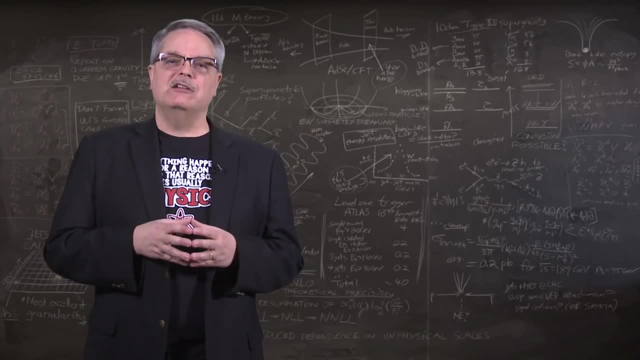 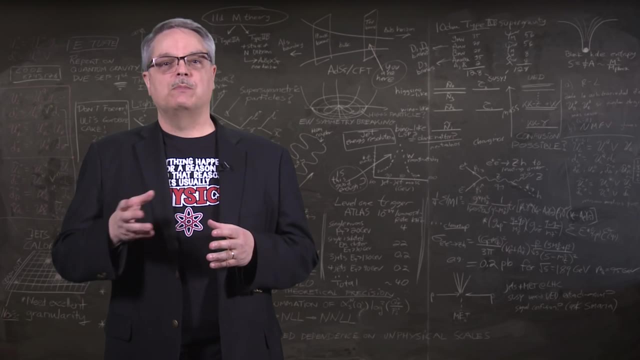 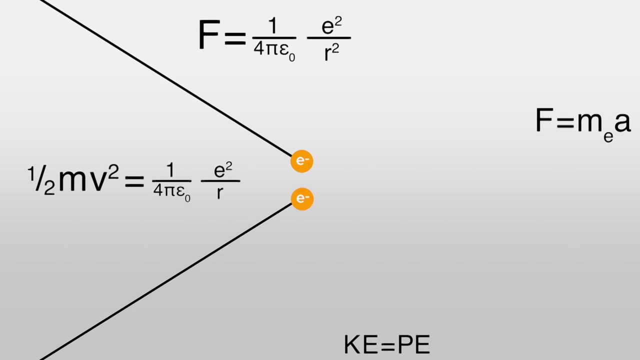 a high-energy particle collision. Feynman's diagrams are easy to write and easy to understand, at least at the most basic level. For example, let's talk about the simplest particle collision imaginable, when two electrons bounce off one another. Classically, we'd calculate this process using the electric field and considerations. 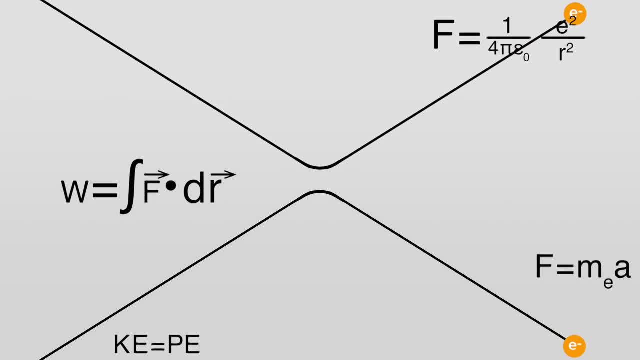 like conservation of energy or just a smidge of calculus. However, in the quantum world, we need to remember that not only do electrons come in discrete chunks, but so do photons. In fact, a form of photons make up the electric field. So maybe when two electrons scatter, 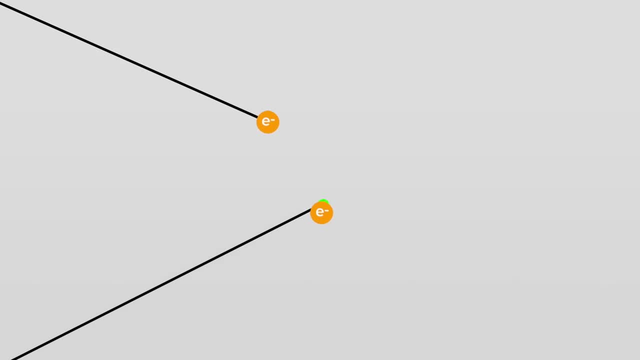 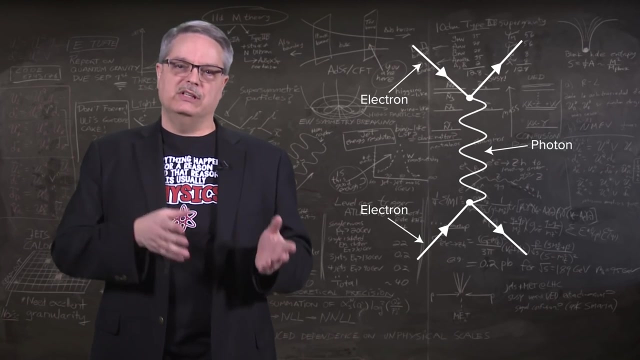 they do so by two electrons approaching one another, and then one of them emits a photon, which then hits the other electron. Both electrons recoil using the standard energy and momentum physics you might have encountered in school, So we can draw the Feynman diagram that does precisely that: Two electrons exchanging a. 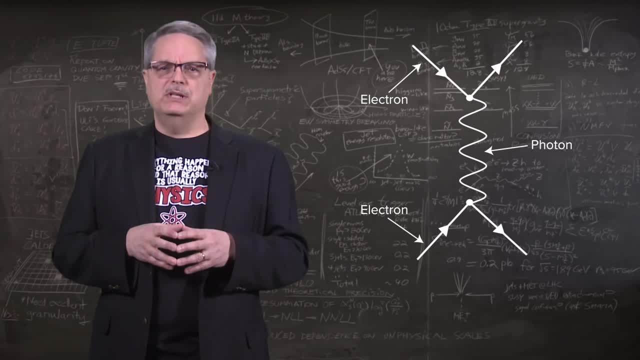 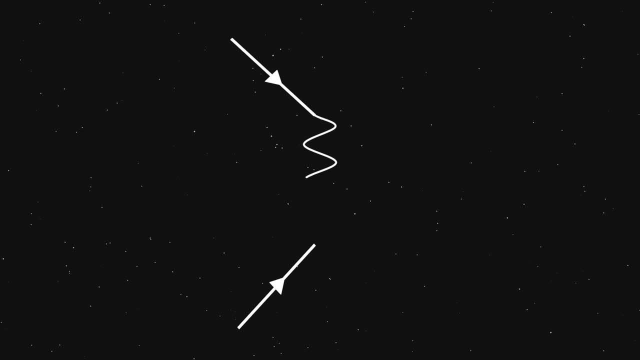 photon. Easy right, We're going to focus on this particular Feynman diagram, but you should know that there are others. For instance, another way in which two electrons can scatter might be that one of the electrons might also emit an additional photon, either before the big scatter or after. 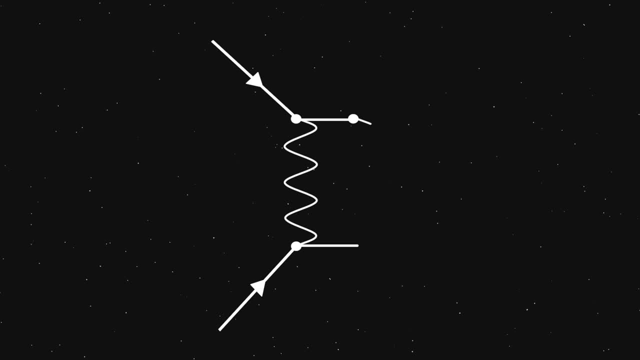 There are other options. For instance, maybe one of the electrons could emit a second photon that is absorbed by the other electron. Or maybe an electron could emit a photon that it then reabsorbs. Or maybe, as the photon moves from one electron to another, it might temporarily turn into 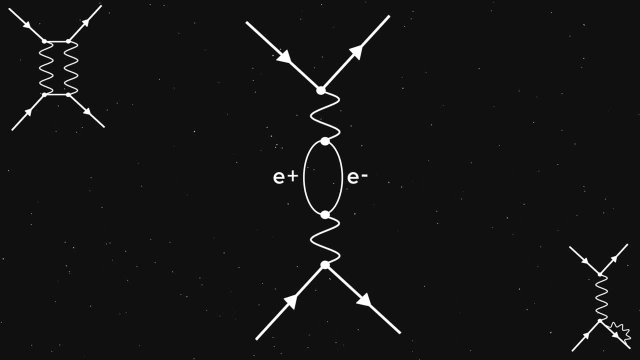 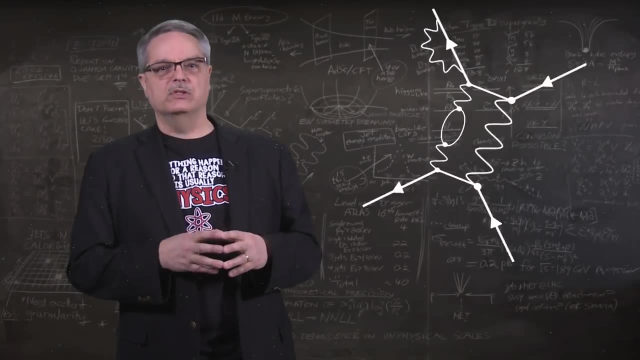 an electron-positron pair before it recoalesces into a photon to complete the scatter. Or we could imagine something even crazier still, with multiple photons being exchanged, with some of them creating other particles and the photons interacting with the temporary particles. There are tons of possible combinations of particles and 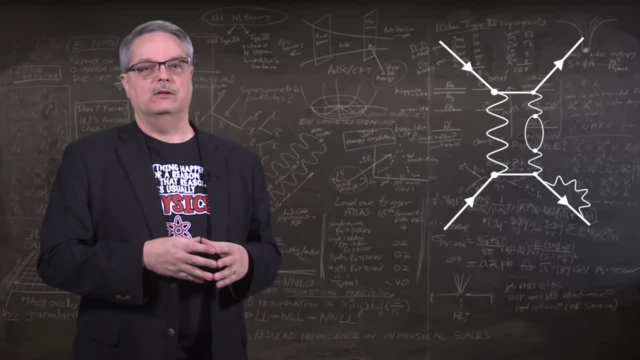 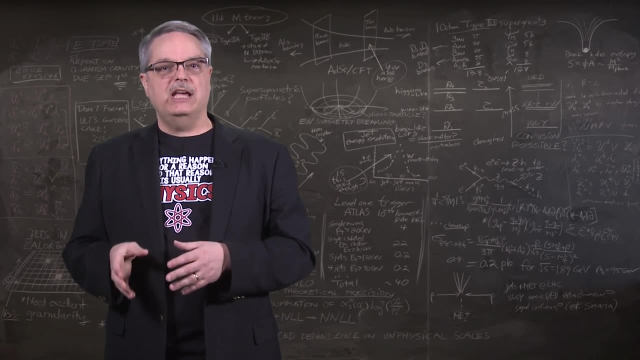 the result is the same basic outcome, which is that two electrons scatter. While all things could happen, it turns out that each time a photon interacts with a charged particle, the chance that this happens is less and less likely, And that's a big effect. 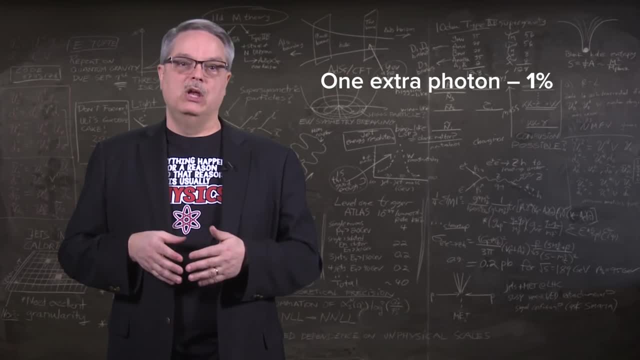 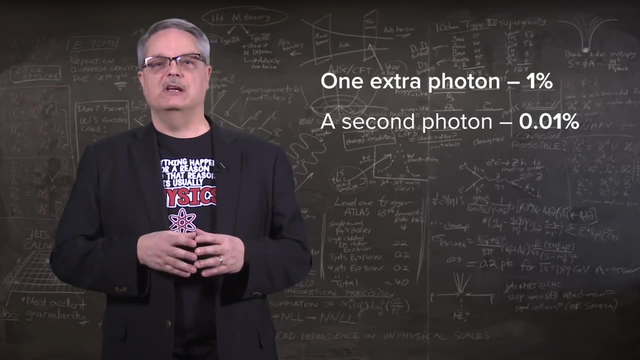 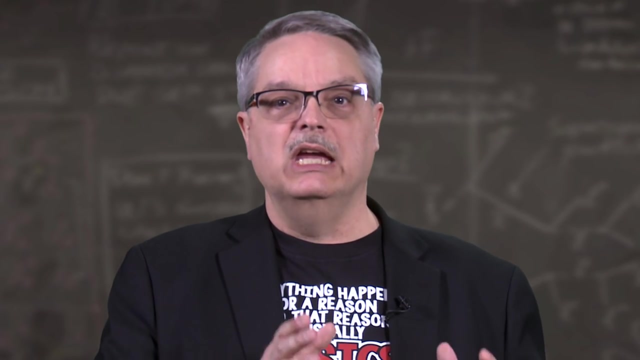 A single extra photon emission drops the probability to one percent, while two emitted photons drops the probability to one percent of one percent. So really only the one simplest Feynman diagram can do that, And this is a crucial point. The single photon exchange is the dominant contribution and 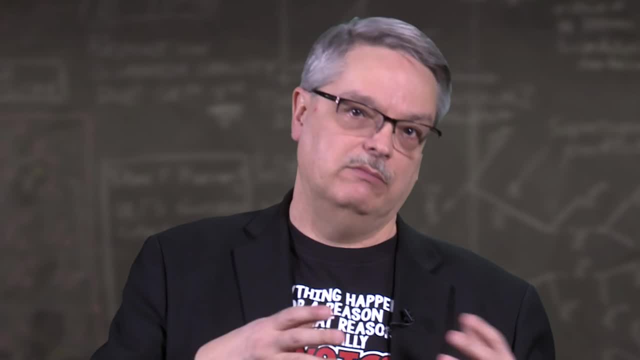 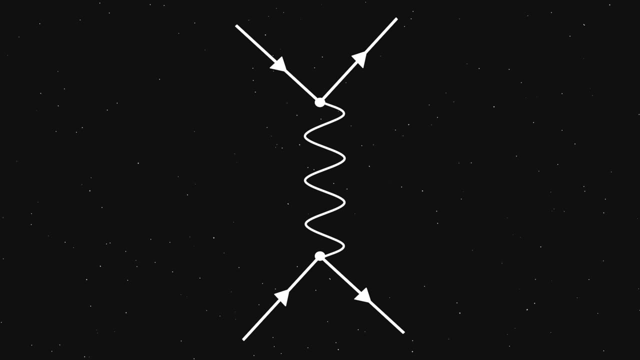 only for very precise calculations do you need to take into account the other diagrams. Let's return to the case of a single photon exchange. So what does that picture tell us? Well, I'm going to say something that might just blow your mind. The picture is really. 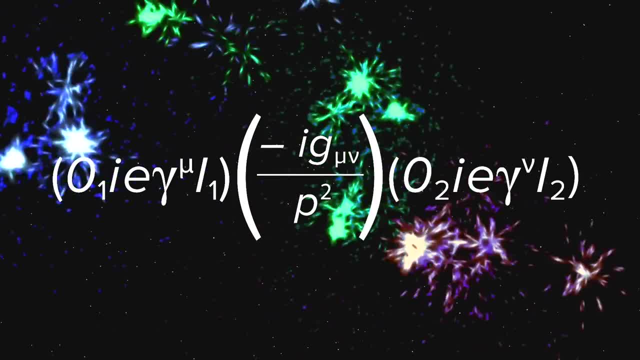 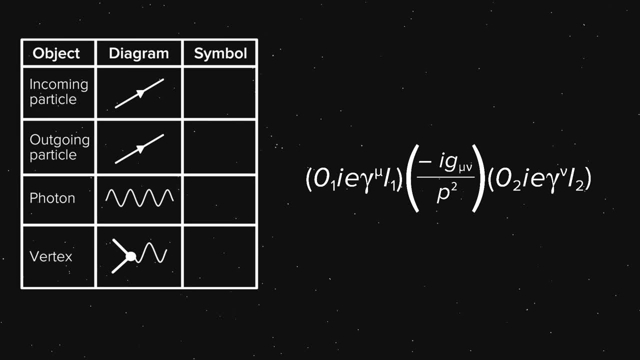 an equation. Now to understand that, I'm going to guide you through the pieces, starting with the vocabulary. Each symbol in the picture corresponds to a piece of an equation. For instance, the incoming electron corresponds to the letter i, while the outgoing electron 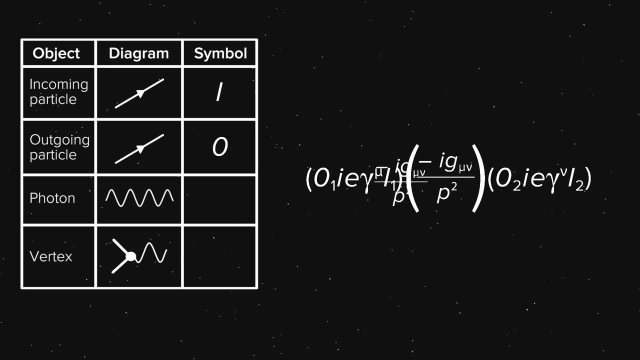 corresponds to the letter o. The photon corresponds to a fraction, specifically minus i g sub mu nu over p squared. The i is the square root of negative one, while the g sub mu nu is used to handle adding up all the relevant subatomic spin for the photon. The p is just. 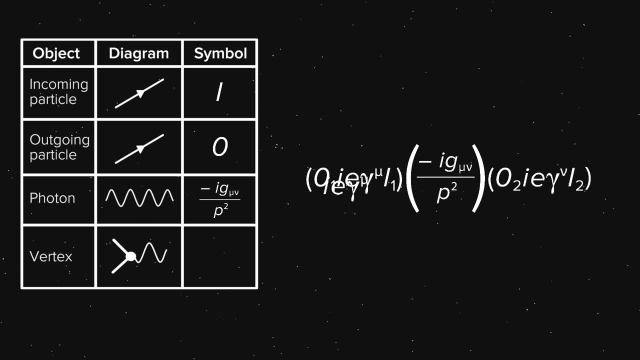 the energy carried by the photon. A vertex has its own corresponding mathematical term, which is an i, e, gamma, where the superscript mu or nu doesn't mean a power like squared or cubed. Instead, it has some implied information on how to add everything up and is related to the subscripts in the g from the photon.